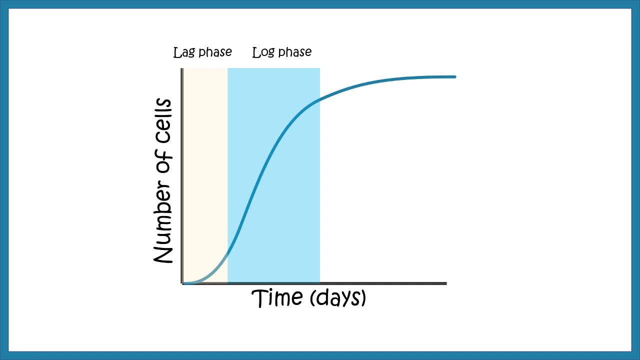 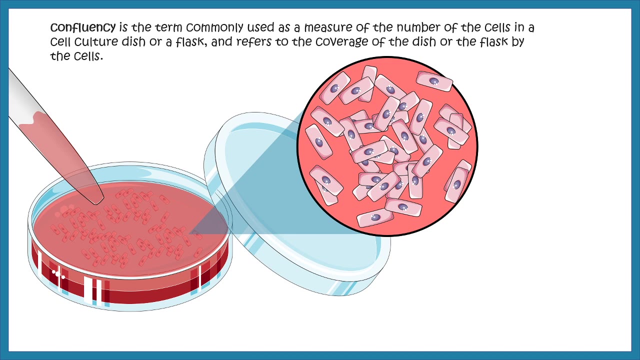 grow, the media gets limiting and also there is not enough surface area for growth. So all of these factors leads to a plateau phase. So whenever a cell culture or whenever a cultured cell reach these plateau phase, you would see this is termed as confluent cells. Confluency is commonly used as a measure of 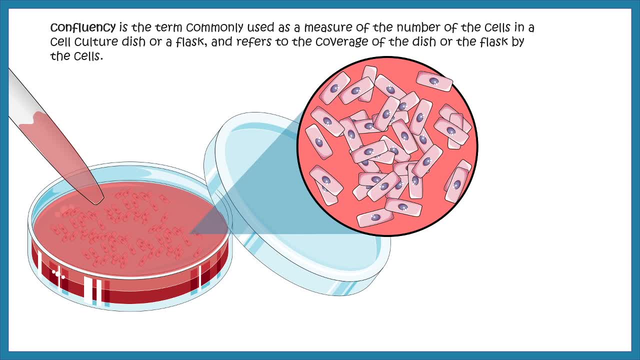 cell numbers, and I mean cell surface area versus the surface area of the culture dish Just to get an idea that how much crowded these cells are. If it is too much confluent then it won't get enough amount of media or necessary nutrients for its growth. So when they are super confluent then you 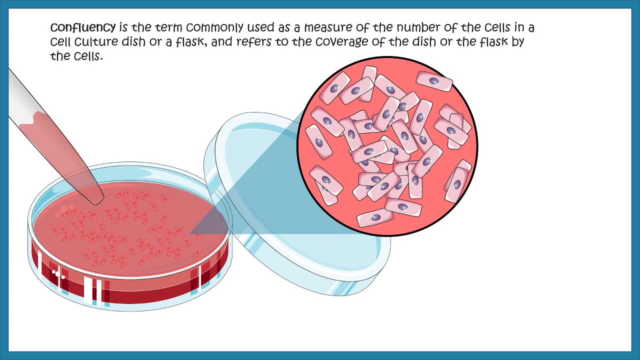 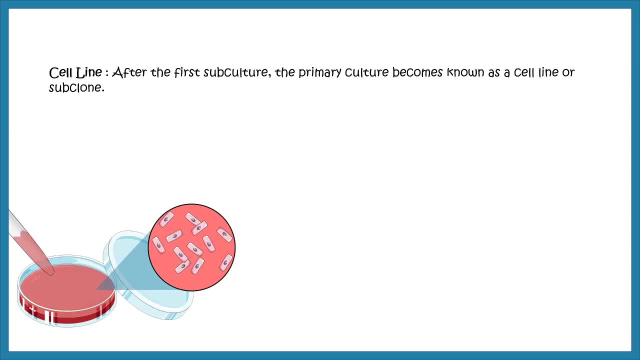 need to sub culture them, and first time you subculture from these cell types then they would be known as a cell line. so cell line is just a subclone which is derived after the first subculture. so from this culture, you see, these cells are now confluent. it's time to separate them into two different hubs. 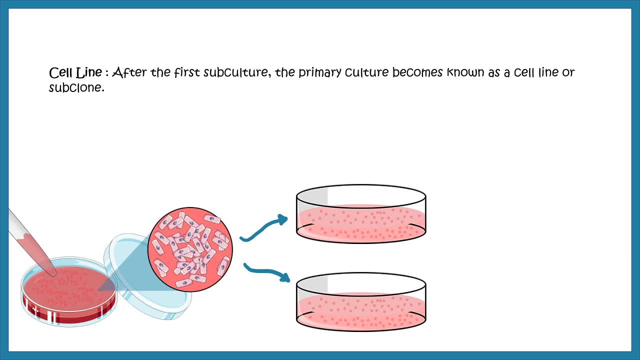 and we term it as subculture. so after subculturing it would be termed as a cell line. now cell line which is derived from a primary culture have limited lifespan and as they are passaged, many cells which are having highest capacity of growth, they predominate the culture. 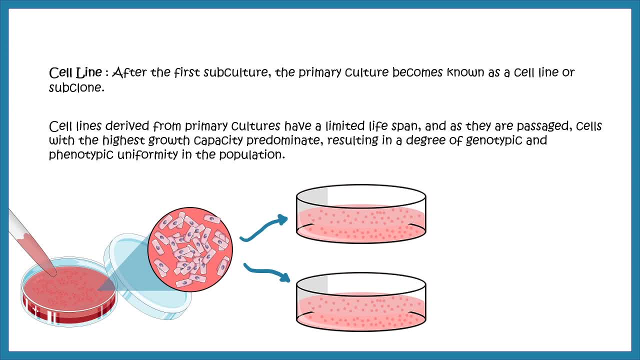 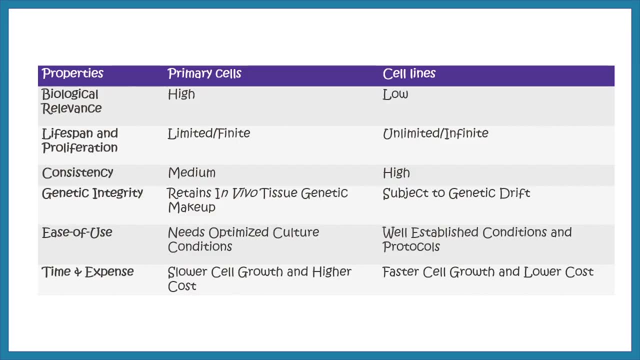 so this results in a high degree of genotypic and phenotypic similarity or uniformity in these cell cultured or in this cultured cell population. so let us quickly compare the properties of primary cells versus cell lines. so obviously i would say the primary cell has a very high biological relevance compared. 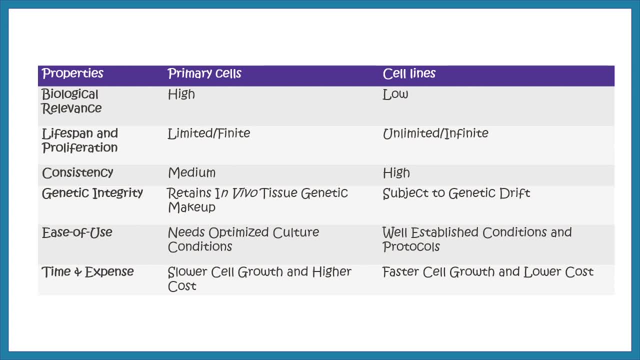 to a cell line. i'll tell you why in a moment. but if you talk about the lifespan, both could have sort of like the primary cell could have like a limited to finite lifespan where cell lines are generally infinite or unlimited. now there are many other points where they differ, but these primary 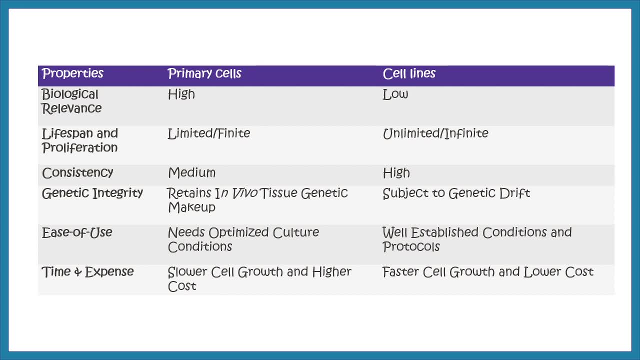 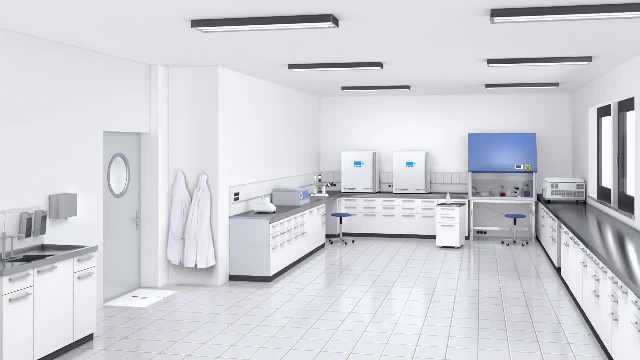 cell culture recapitulates the tissue-like organization way more than the cell lines. i'll tell you why, but before that let's try to understand this process in a lab setting. in order to understand cell culture, we have to virtually explore a cell culture lab. so here is a cell culture lab. you can see the essential components. it should be very 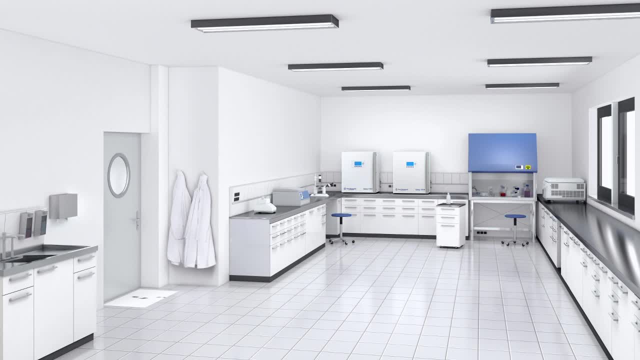 clean and it should be tidy. so in the cell culture lab on the right hand corner you can see there is a biosafety cabinet. all the actions would take place here. before looking at the biosafety cabinet, let us look at other components so you can see just left side of the biosafety cabinet there are 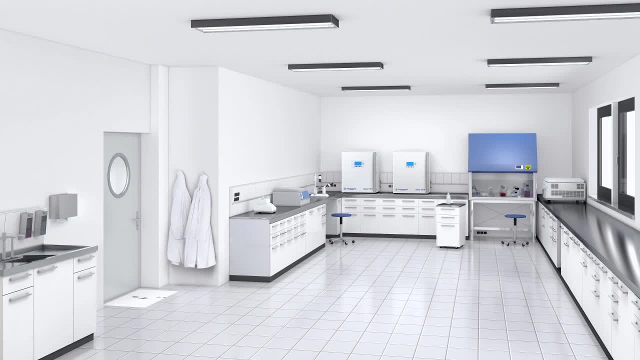 there are two incubators, which are important for keeping the cells, and they would provide the proper environment for the cell to grow. other than that, there would be centrifuges, microscope, cell counter, etc. so there are certain norms that you have to follow when you are working on a cell. 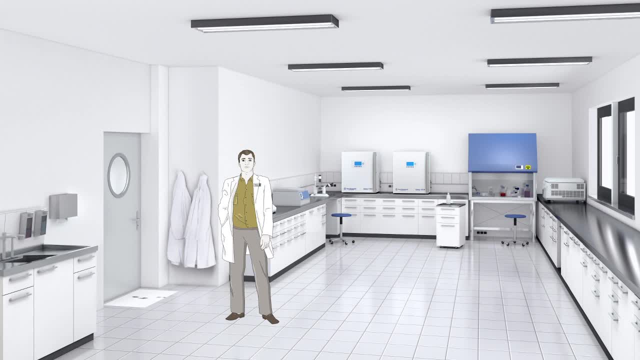 culture lab, such as wearing a lab coat all the time, a covered lab coat, obviously- and if you're culturing something which is infectious or any other, uh, serious material, then you should have a additional layer of protection. you have, you should have your proper ppe kit in order to culture the cells. now, guys, what you need to. 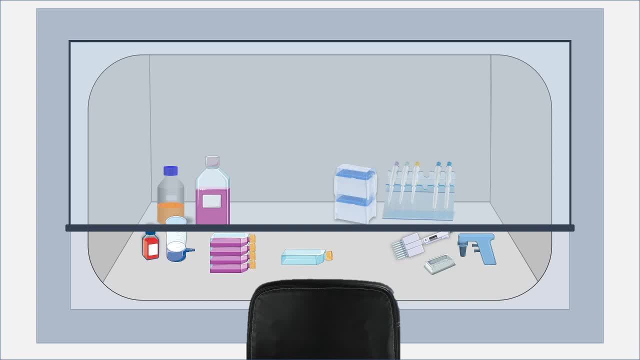 understand is what is inside the hood. these hoods are generally. what is depicted here is a classical bsl2hood or biological safety level 2hood. however, biological safety level 3 and safety level 4 hoods are very dangerous. bsl2hood or biological safety level 2hood. however, biological safety level 3 and safety level 4 hoods are very damaged. 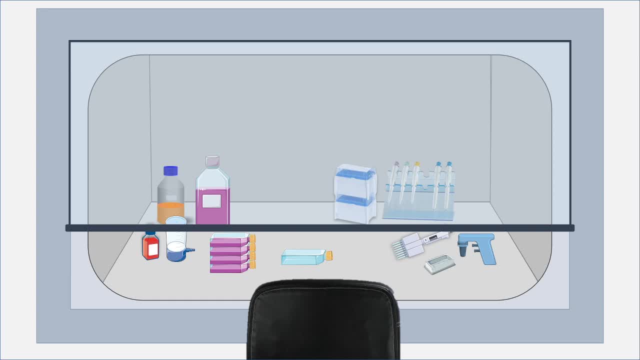 and you have to buy a nunchuck because the natural material, which include particle, can be easily broken and nevertheless finalized by anyone. biological safety level 3 felt free to practice a nunchucks and other resources, including physical, different looking and other videos will talk about that, but not in this video, so you can see there. 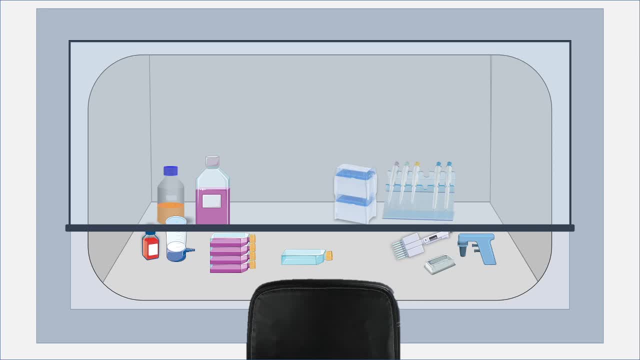 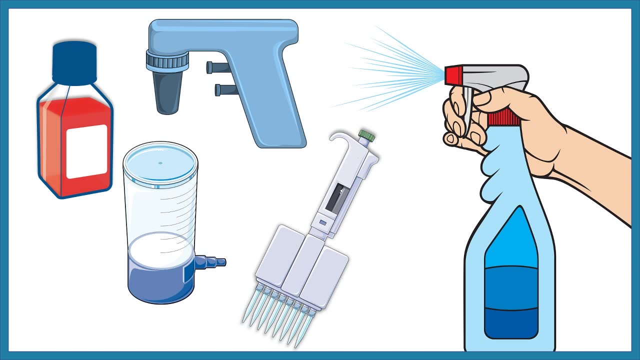 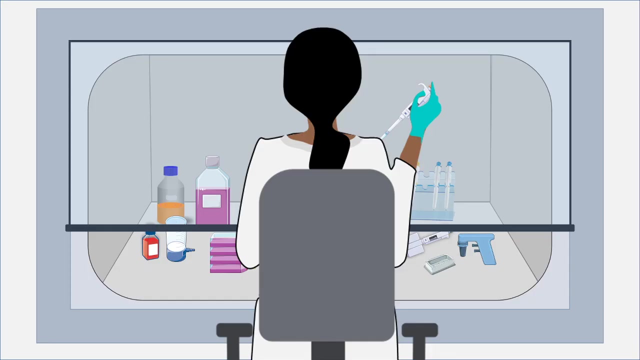 are many things which are associated with cell culture- should be placed in the hood, but it should be first sprayed with alcohol and then it should be kept inside the hood such that it is contamination free. now, while working in the hood, it is always permissible that you wear lab coat, and having 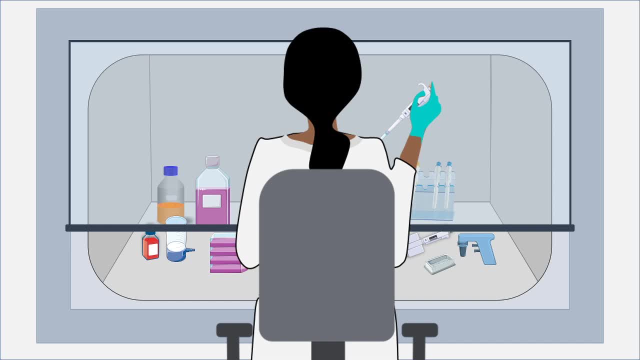 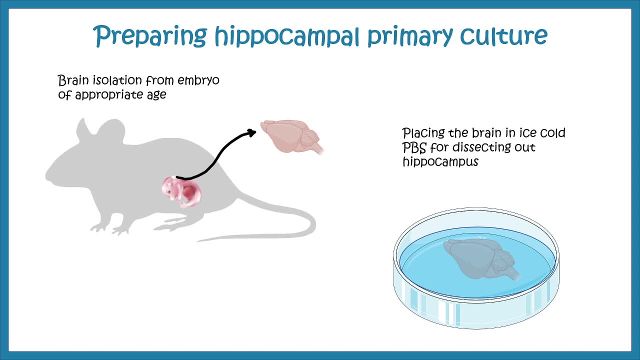 proper gloves and other protective equipments. this would prevent contamination and also save you for from any kind of biohazards. so let's try to understand how we can prepare a hippocampal primary cell culture, just to get an example. so, in order to culture the hippocampal neurons, we 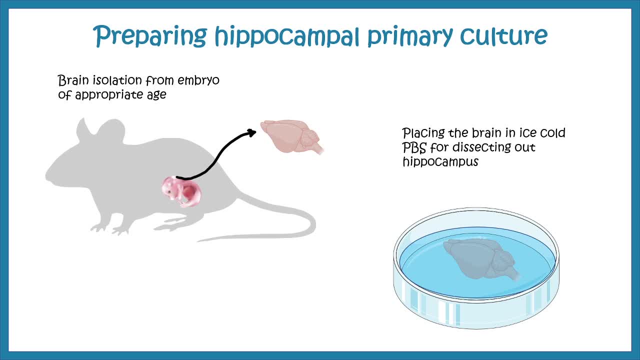 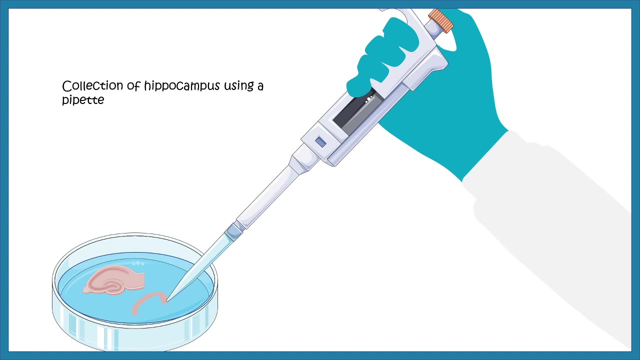 need to isolate brain from mouse generally in lab mouse are available right, so you can take mouse embryo out and take out the embryonic brain in a ice-cold PVS machine solution. now, after dissecting these brain in an ice-cold solution, you dissect out the 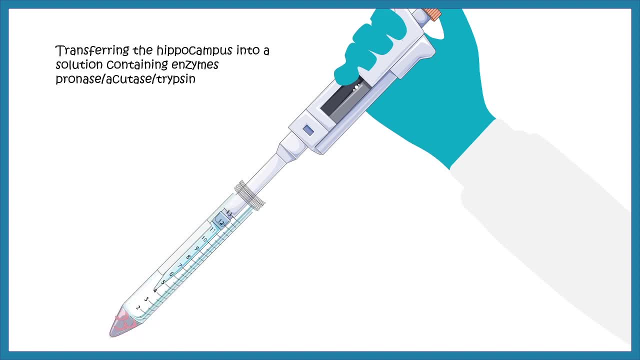 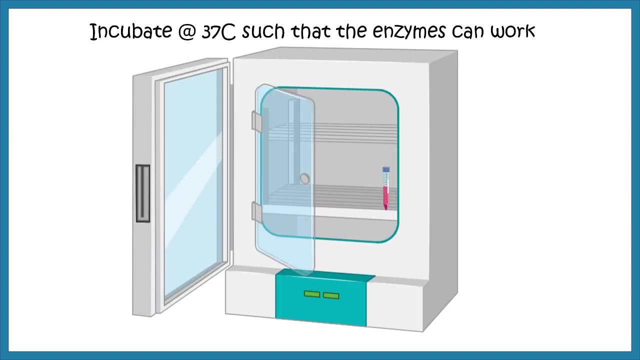 hippocampus and collect it in a particular tube containing trypsin, acutase or pronase. so all of these enzymes are able to dissociate these content of this tissue. so all the cell types which are present in that tissue would be dissociated now. so obviously you put it in. 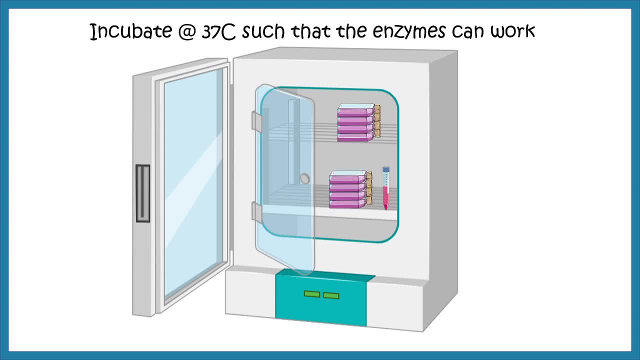 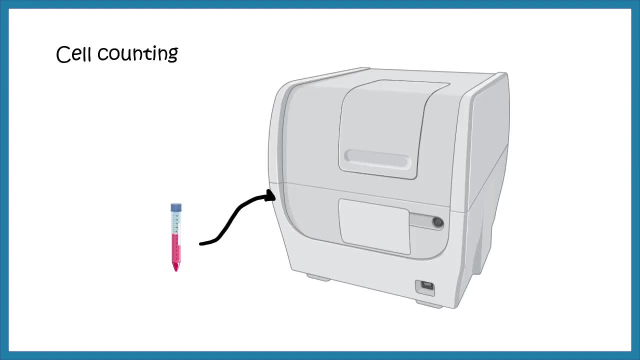 the incubator for some time, such that the enzyme can work, and after that you pipe it up and down vigorously such that it creates a cell suspension. now, after that, it is necessary to count the cells to get an estimate how much cell you need to plate in a culture- roughly about a. 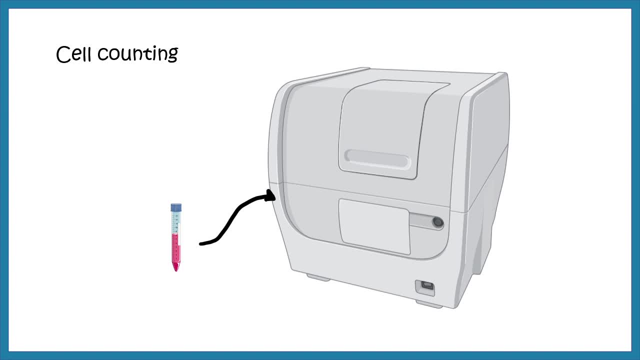 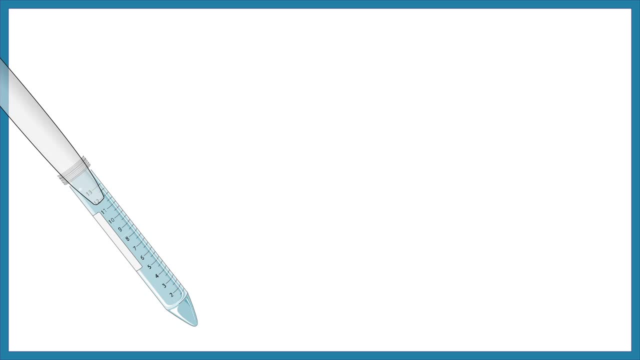 million or 1.5 million cells are a good material to start with, and it also depends upon flux, volume, volume or kind of a container where we are culturing the cell. I just talked about a 10 centimeter plate now. after that, you resuspend these cells in the media. 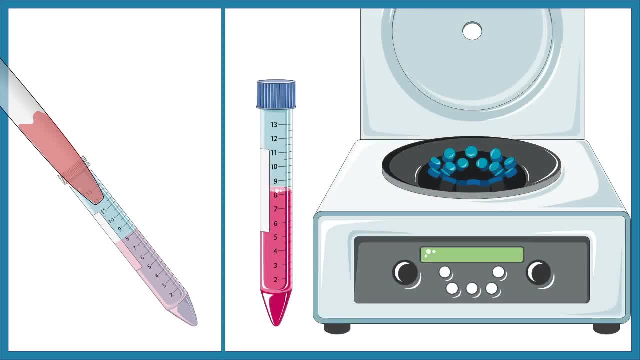 cell suspension. you, you make a cell suspension in the media and then what you have to do? you have to centrifuge them and wash them, because the trypsin which is already there in that media would be harmful. so you need to get rid of these trypsin. so supernatant is discard, whereas the 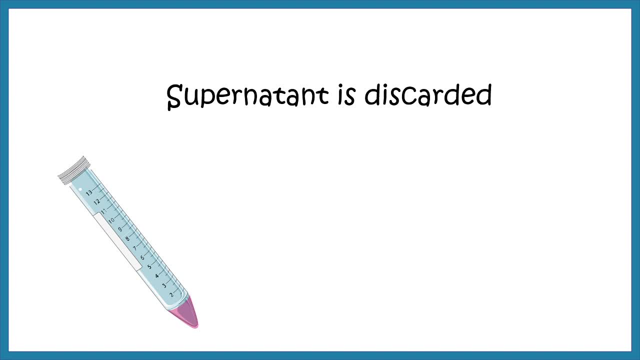 pellet of cells is retained after the trypsin is gone. then again, the cells are washed with PBS and ultimately resuspended with the culture media. now, this culture media which we add, we pipe it vigorously in this step to mix our cells, to break the clump of cells. 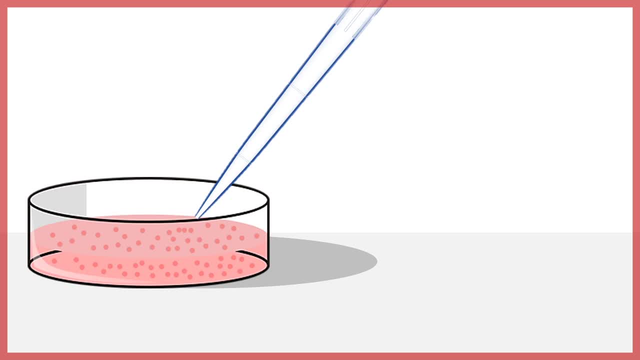 and make them a suspension, and finally, we plate them in a 10 centimeter plate or whatever plate that we have in supply, and this is how we establish a primary culture. now, all this thing is just in a animated fashion, right? so let's look at this process in bit more details. 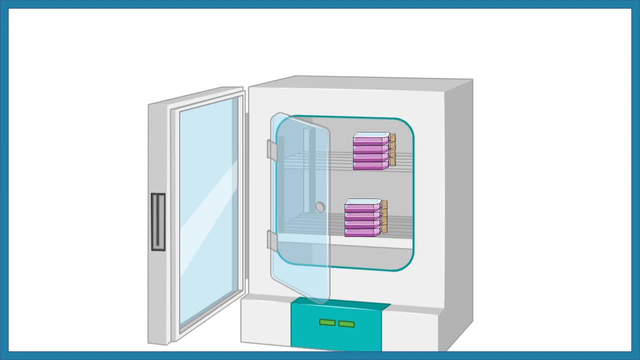 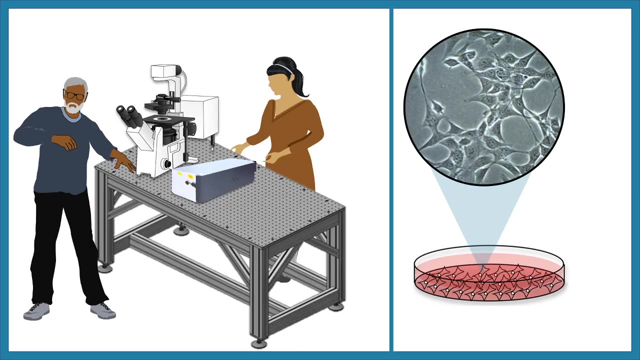 in a realistic setup. so ultimately you put it in a incubator for their growth and monitor them almost every day and change the media every alternate day and lastly, you have to check it in the microscope right to check their growth. in this case, you can see these neurons are taking. 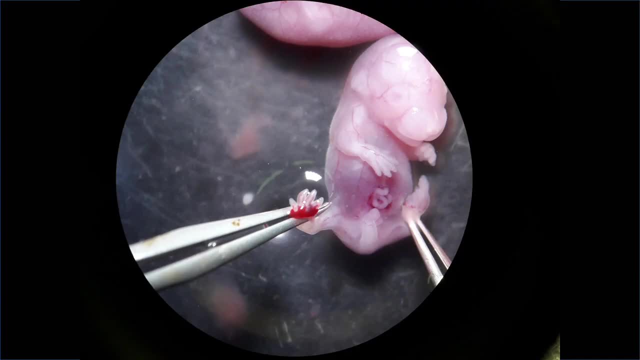 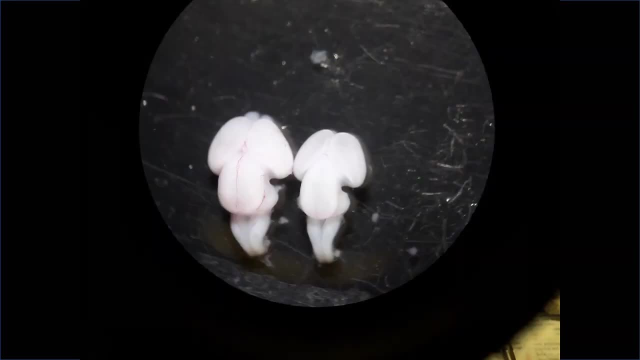 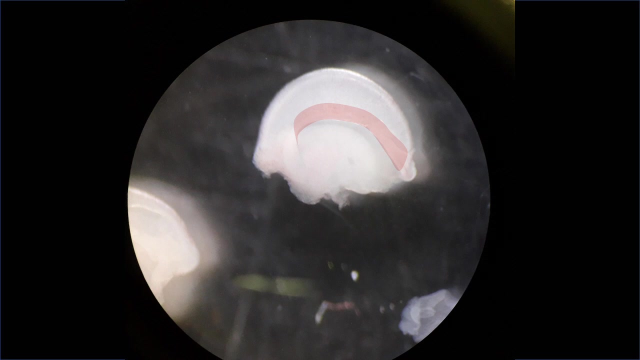 their shape and forming connections in this culture. so let's look at the original process. so here you can see a mouse embryo and then you can dissect out the brain like this, and from a. from this brain you know where the hippocampus is situated, so you can micro. 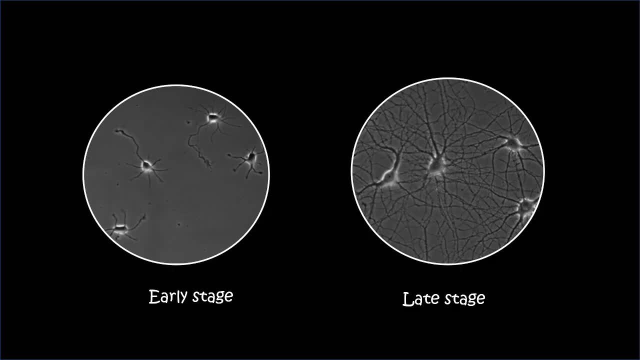 dissect this hippocampus and culture them, and in a culture setting at a very early stage you see hardly. they have new rights and projections and connection in between them, whereas at the late stage you can see quite a lot of connection has been formed inside them and if you track their 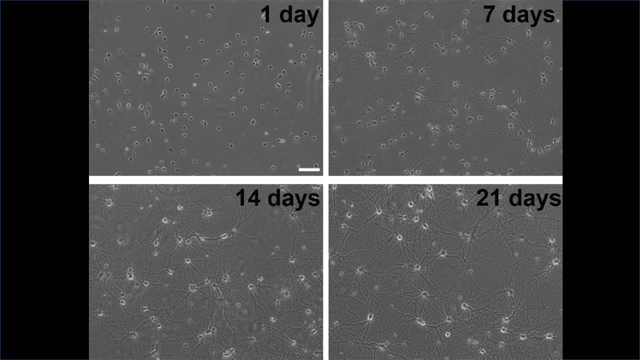 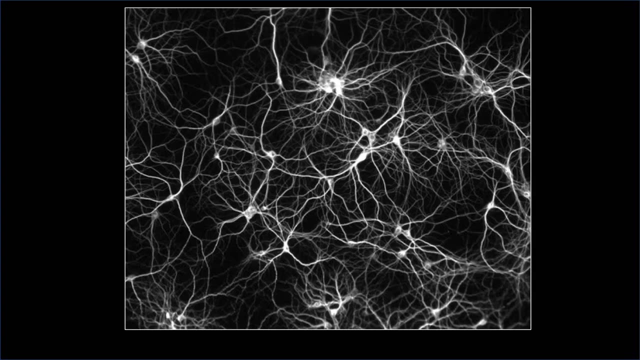 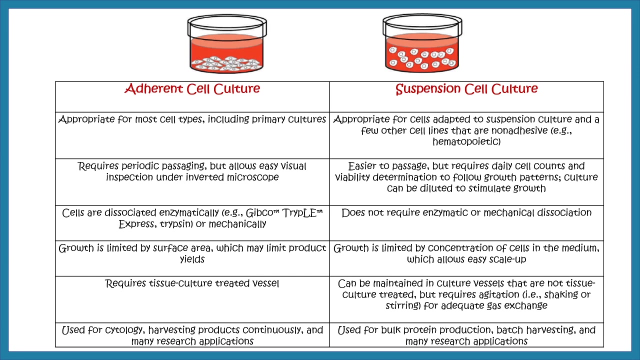 progression over days, you would appreciate how, in the culture setting, they are growing and forming connections with each other and making a functional Neural Network. so obviously this is a mature Neural Network, which is depicted in this image and courtesy, of course, Google images. now let us talk about two different type of cell culture paradigm. one is known as adherence cell. 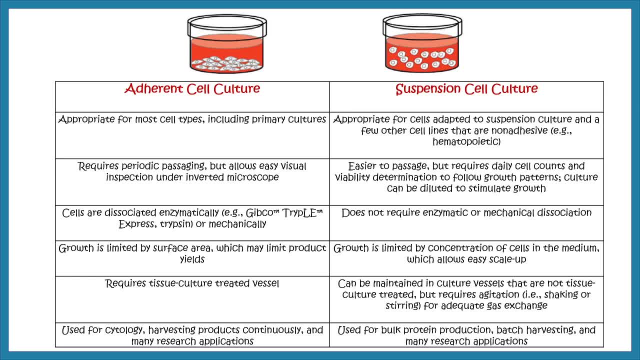 culture. another is suspension cell culture. so adherence cell culture is basically what the cells get adhered with the plate material. generally, the plate need to be coated with some kind of extracellular Matrix proteins, such as lamin fibronectin, sometimes such that these cells get them on which they can grow, whereas many cells don't need this substrate of our group. imagine. 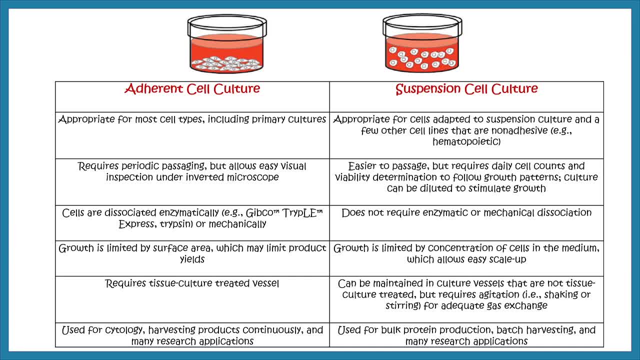 a blood cell. obviously in an in vivo setting they are floating here and there. so obviously in a cultured setting they can also float. so obviously it's easy to handle a suspension cell culture than adherence cell culture and it's easier to sort of like sub culture them and a lot of 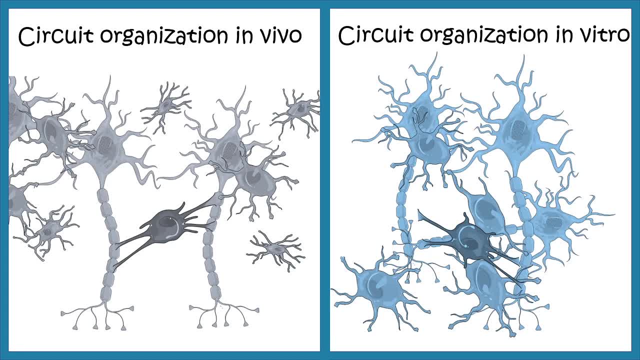 difference has been noted here. now let me tell you why these culture systems are not so good. these culture systems have some advantage but a lot of disadvantage. imagine you have a circuit organization in vivo in a certain fashion, so certain amount of glial cell is connecting a certain amount of neuron in a specific stoichiometric ratio. that ratio, that 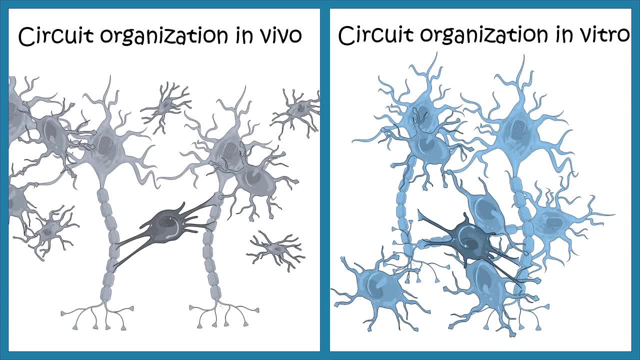 organization, cellular connection. these might be totally jumbled up. when you are culturing, because you are first breaking the way of connection formation and then you're allowing it to be, so, exactly the rules or the micro environment in which these connections form would be very different. that means, though, culture settings can allow the cells to be grown in vitro, but they have 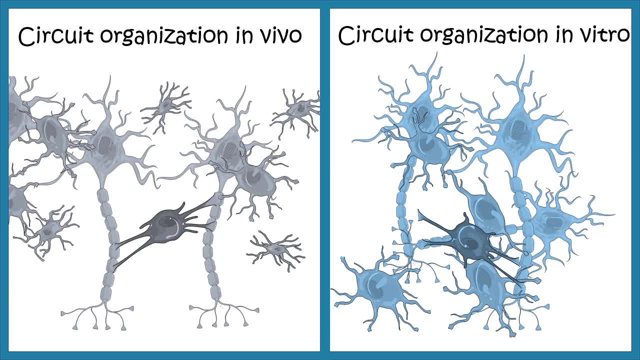 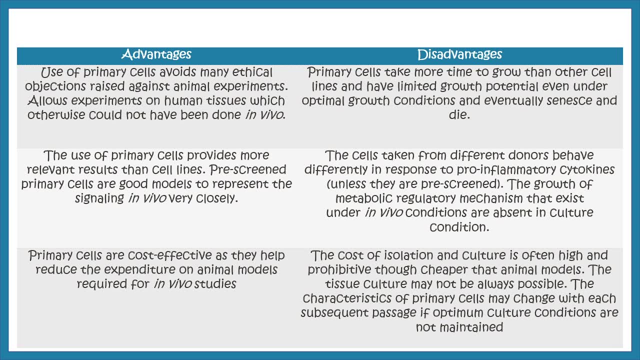 a lot of limitation. as a researcher, it is really important to understand the limitations, such that we can design our own experiments right. so obviously we have certain advantages, such as: like the primary cell cultures, they are more closer towards the in vivo settings than a cell line, because cell lines sometimes there. 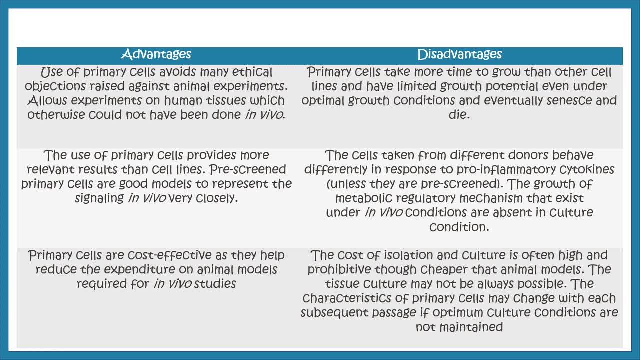 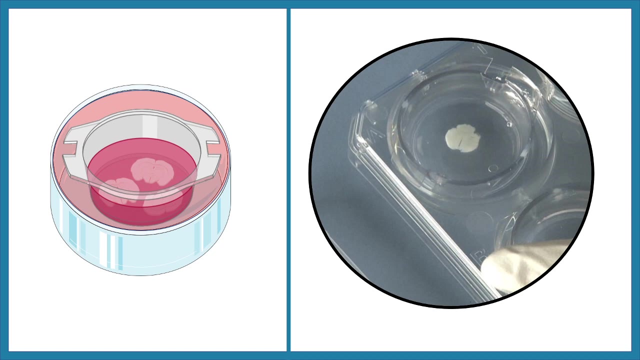 are chromosomal aberrations, there are growth related problems. so really we have to understand what kind of issue we want to chase in this cell, in this cell culture paradigm. based on that, we would use our cell lines, either a primary one or a cell line right. so I hope that was comprehensive enough, but many of the people stopped using this dissociation. 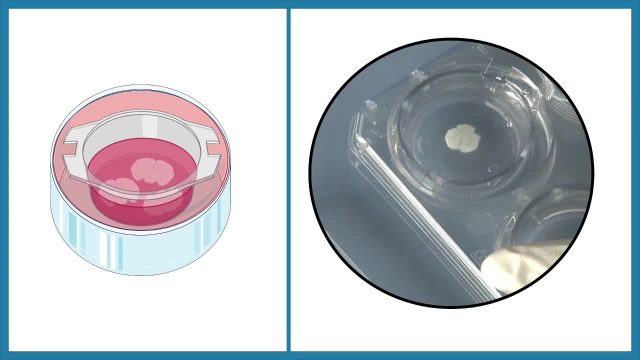 culture method these days the primary culture method. instead of that they started using organotypic culture. so it's impossible to culture the brain in total. but if we slice the brain, then these thin slices can be cultured because nutrient can reach inside, but whereas in an intact brain it is very 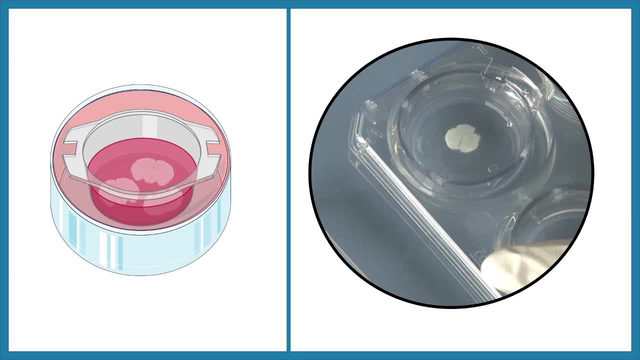 difficult for the nutrient to flow deep inside the brain and that is why there would be necrosis. but in these settings a large surface area is in contact with the culture media, so all these neurons would get some amount of culture media to thrive and that is why organotypic culture is a very good 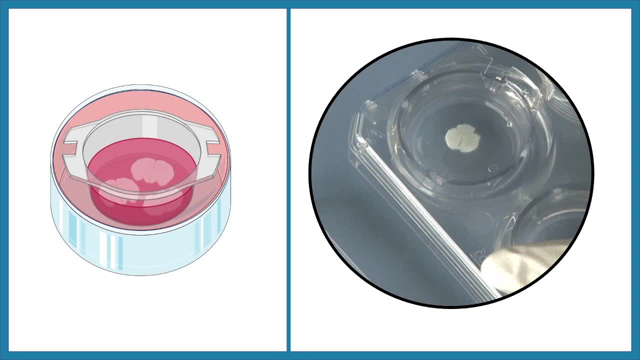 culture system these days and a lot of researchers are using these organotypic culture. in a different video we'll talk about organotypic culture, cell culture, media, etc. so stay tuned and watch my channel. if you like this video, please hit the like button, and if you have any queries, please leave them in the comments below. 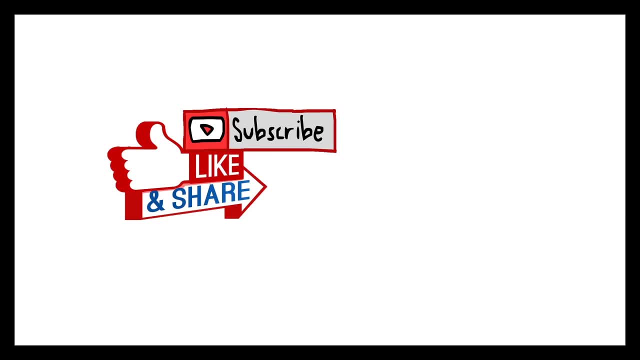 thank you very much for watching and see you next time. bye, bye video. give it a quick thumbs up. don't forget to like, share and subscribe. and do follow me in patreon. you can also be my patreon, just paying only four dollars per month. and, guys, i'm also. 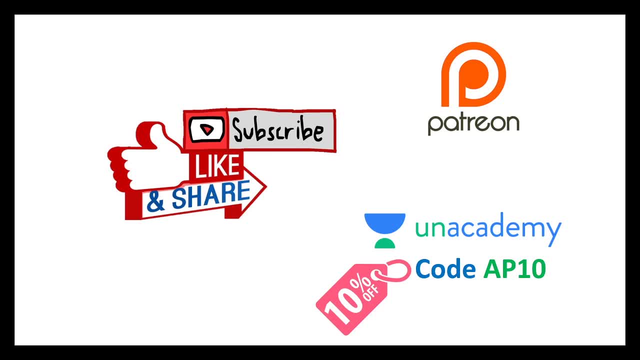 present in unacademy so you can access all of my courses in unacademy. using my code epitane, you would get a 10 discount. so hurry up and thanks for listening. thank you, guys. 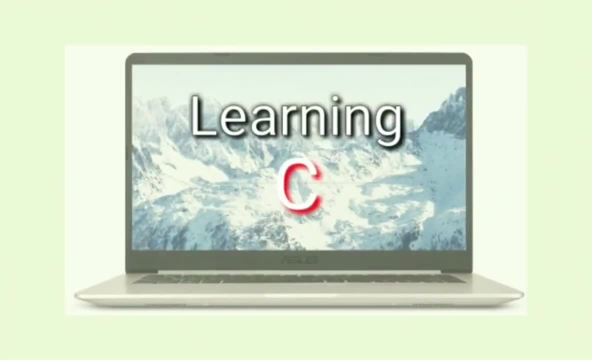 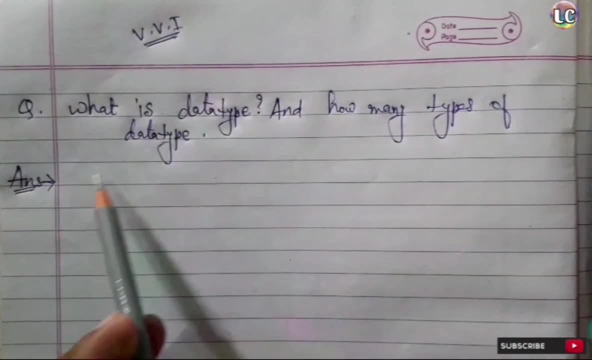 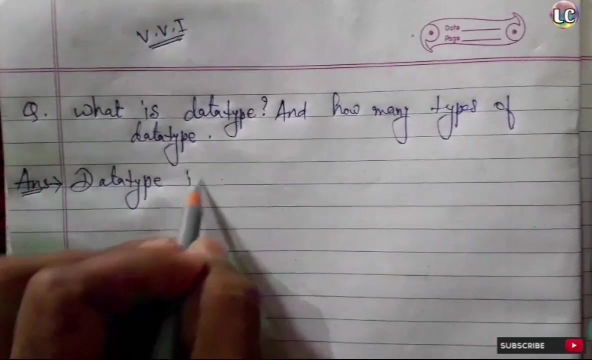 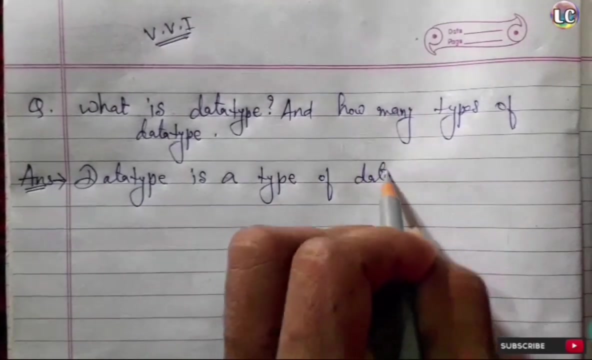 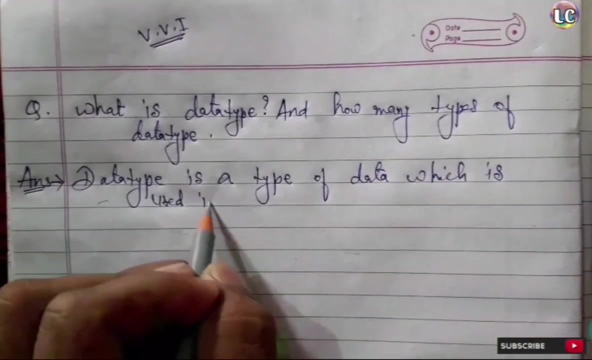 Hi, friends, today I will discuss the topic: what is data type and how many types of data type. So it's a very, very important topic for our syllabus as well as examination. So first of all, we discuss what is data type. So here we write: data type is a type of data. Data type is the type of data which. 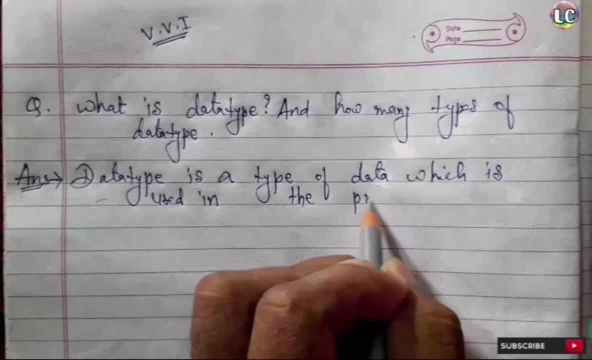 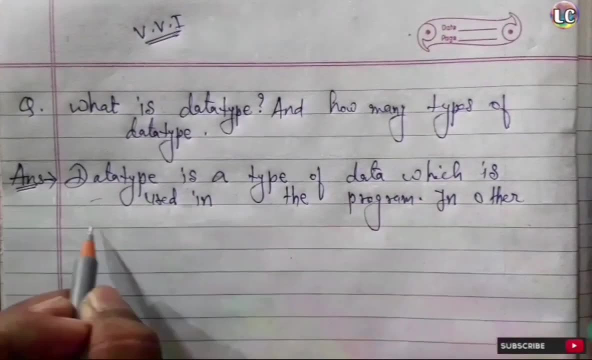 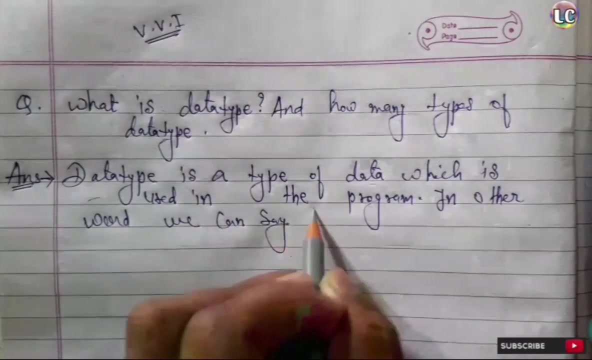 is used in the program, which we use in the program. So here we write: data type is a type of data which is used in the program. In other words, we can say that it is used to declare a variable. In other words, we can say that it is used to declare a variable. 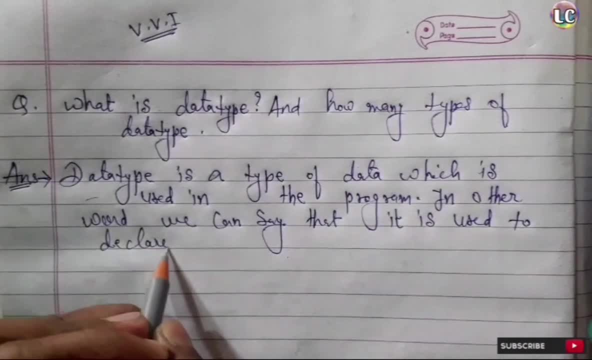 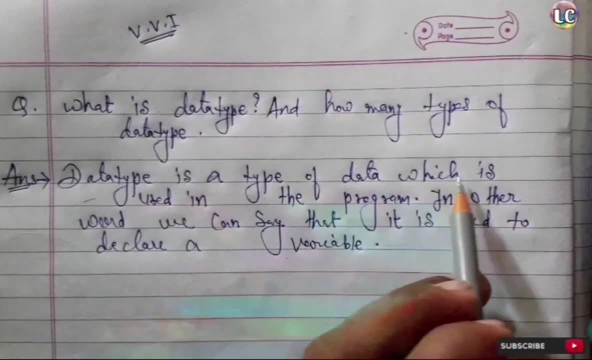 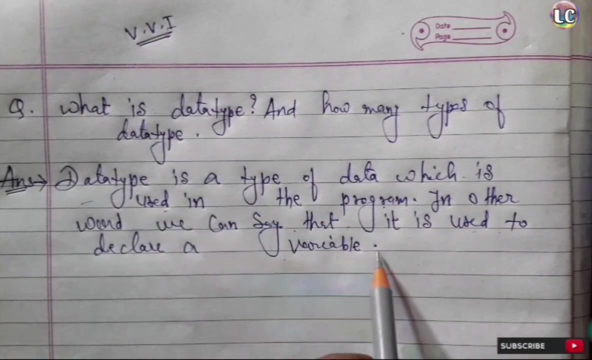